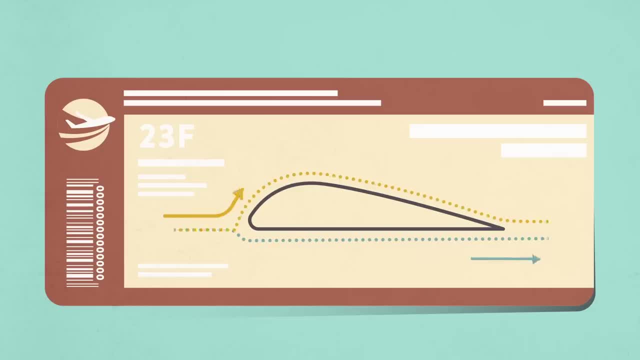 Air molecules flowing above and below the wing don't need to meet back. Air molecules flowing above and below the wing don't need to meet back. In reality, the air traveling above reaches the wing's trailing edge much faster than the air beneath To get a sense of how lift is actually generated. 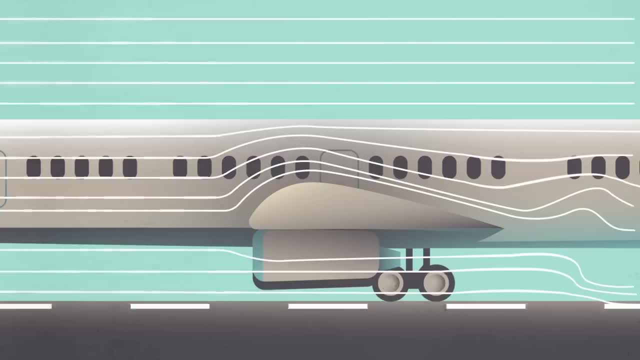 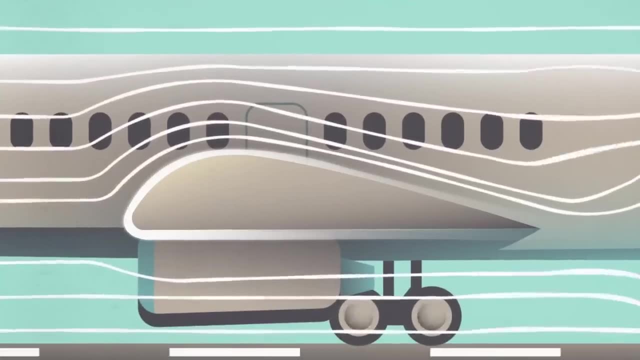 let's simulate an airplane wing in motion. As it moves forward, the wing affects the movement of the air around it. As air meets the wing's solid surface, a thin layer sticks to the wing. This layer pulls the surrounding air with it. 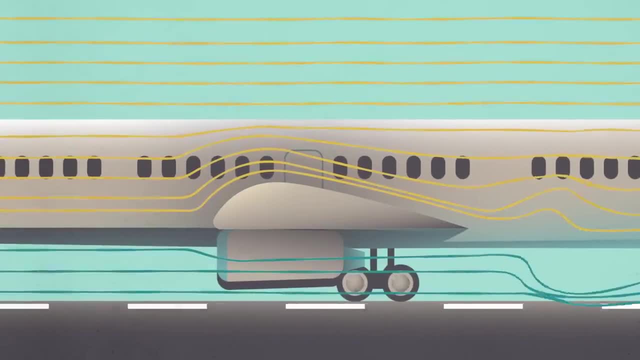 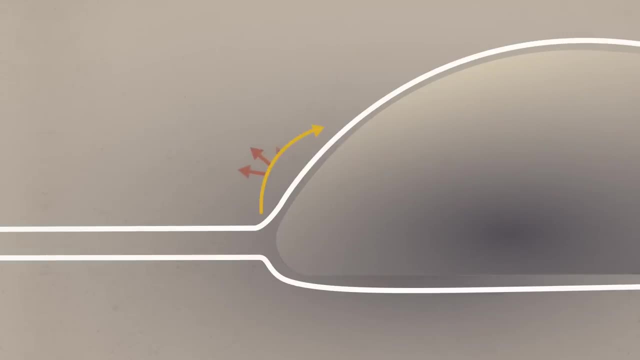 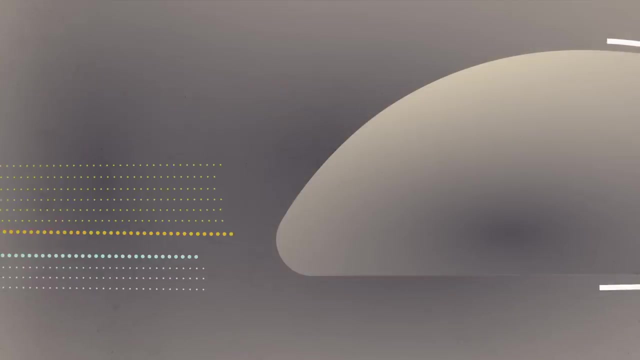 The air splits into pathways above and below following the wing's contour. As the air that's routed above makes its way around the nose of the wing, it experiences centripetal acceleration, the force you also feel in a sharply turning car. The air above therefore gathers more speed than the air traveling below. 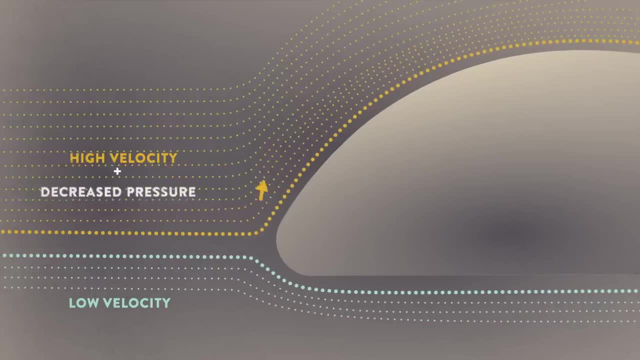 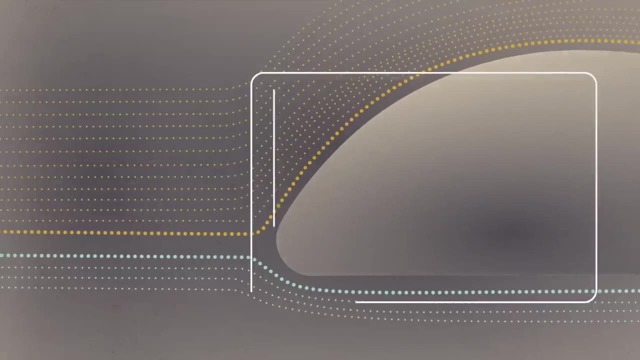 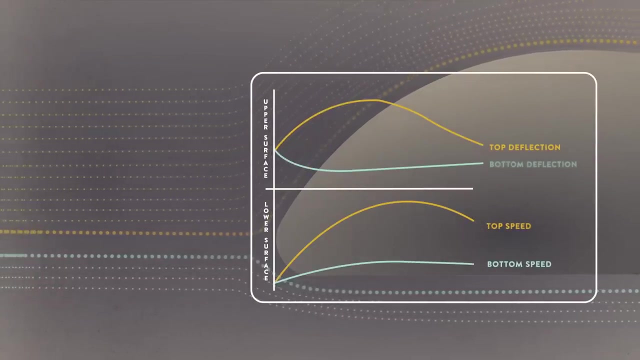 This increased speed is coupled with a decrease in pressure above the wing, which pulls even more air across the wing's upper surface. The air flowing across the lower wing, on the lower surface, meanwhile, experiences less of a change in direction and speed. 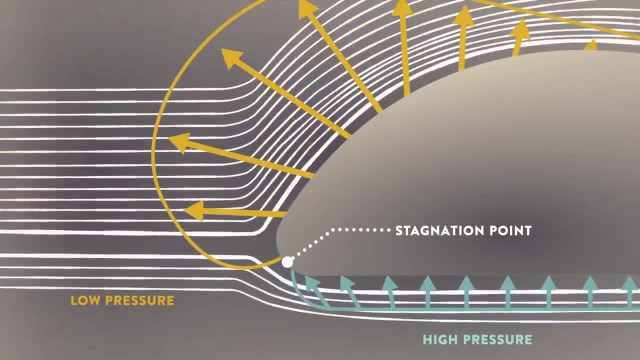 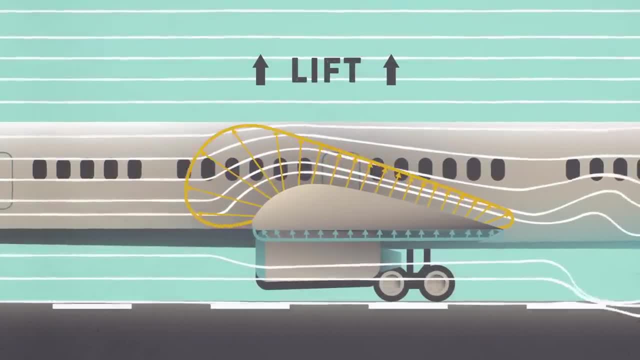 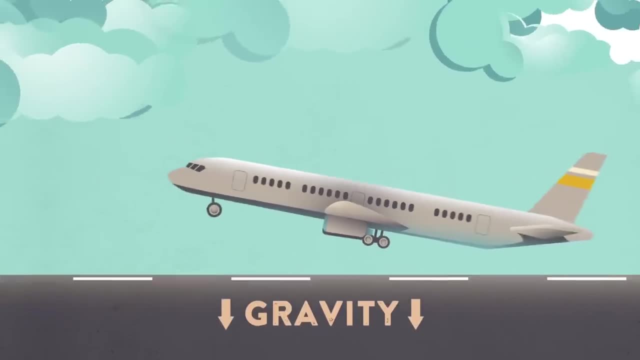 The pressure across the wing's lower surface is thus higher than that above the upper surface. This pressure difference results in the upwards force of lift. The faster the plane travels, the greater the pressure difference and the greater that force Once it overcomes the downward force of gravity. 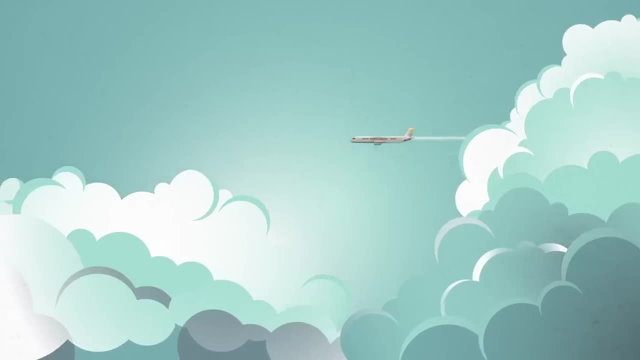 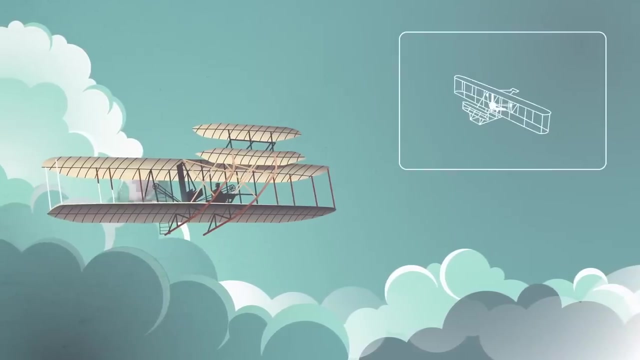 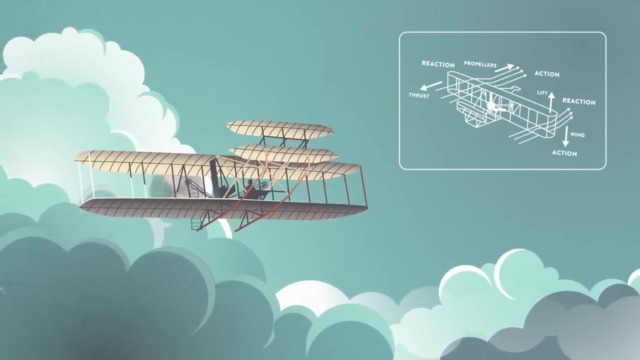 the plane takes off, Air flows smoothly around curved wings, but the wing's curvature is not the cause of lift. In fact, a flat wing that's tilted upwards can also create lift as long as the air bends around it, contributing to and reinforcing the pressure difference. 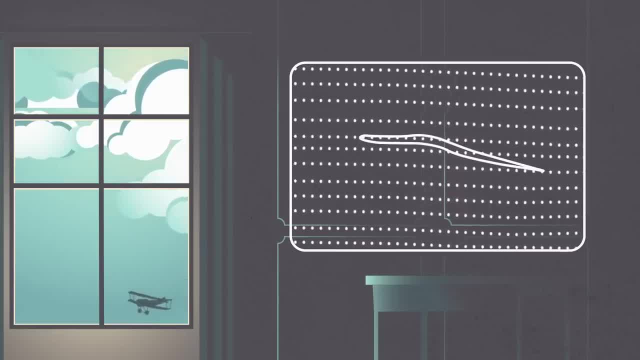 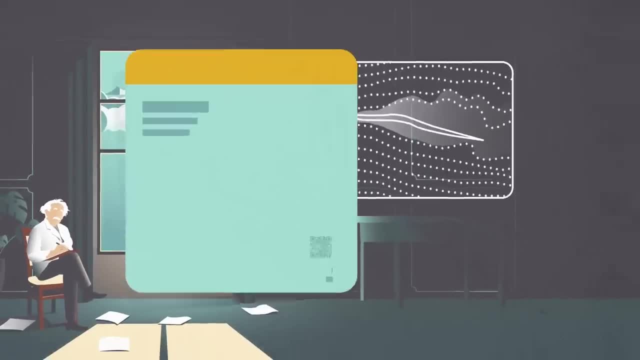 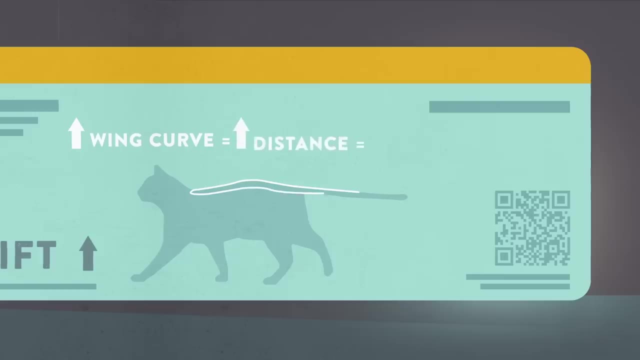 Meanwhile, having a wing that's too curved or steeply angled can be disastrous. The airflow above may detach from the wing and become turbulent. This is probably what happened with Einstein's wing design nicknamed the cat's back, By increasing the wing's curvature. 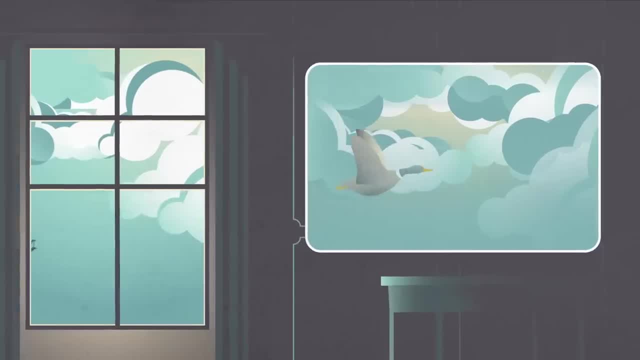 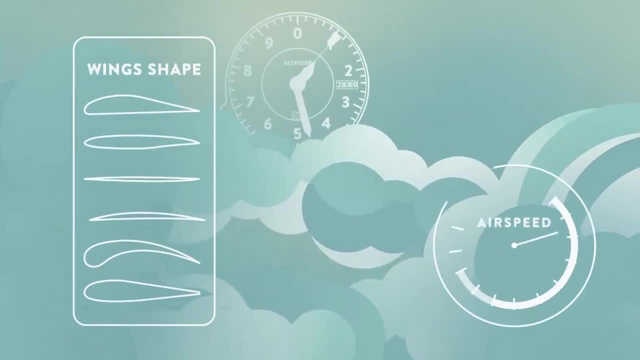 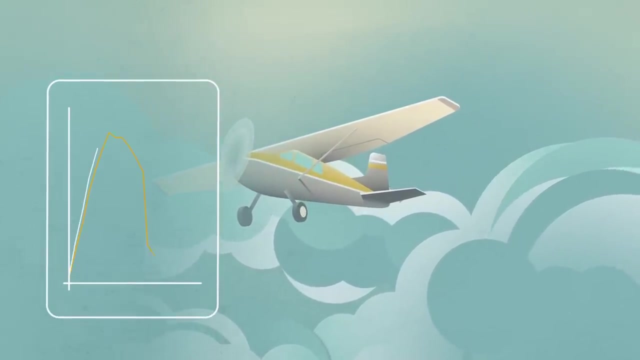 Einstein thought it would generate more lift, but one test pilot reported that the plane wobbled like a pregnant duck in flight. Our explanation is still a simplified description of this nuanced, complex process. Other factors, like the air that's flowing meters beyond the wing's surface. 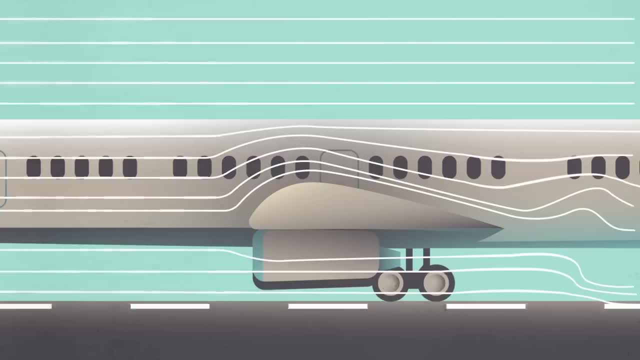 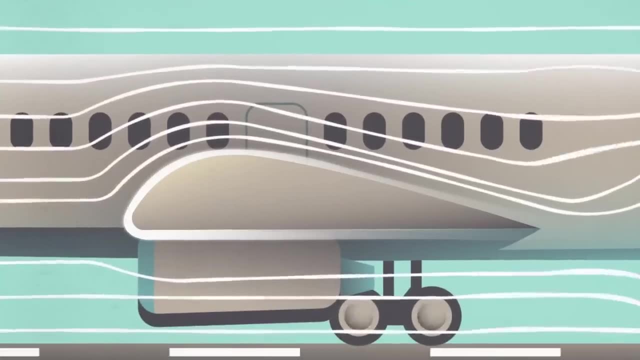 let's simulate an airplane wing in motion. As it moves forward, the wing affects the movement of the air around it. As air meets the wing's solid surface, a thin layer sticks to the wing. This layer pulls the surrounding air with it. 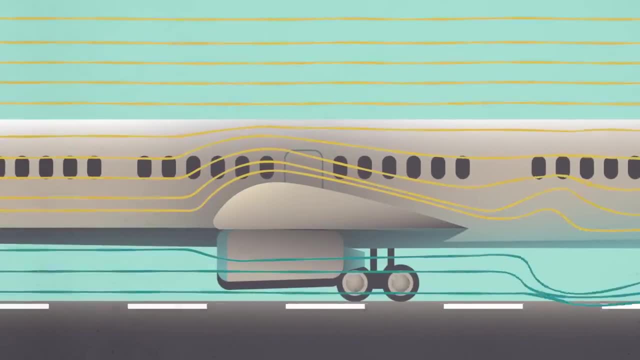 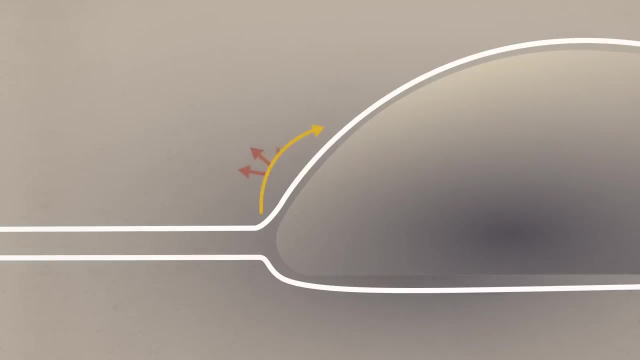 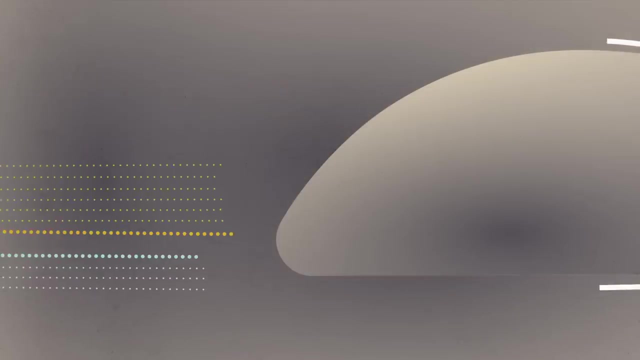 The air splits into pathways above and below following the wing's contour. As the air that's routed above makes its way around the nose of the wing, it experiences centripetal acceleration, the force you also feel in a sharply turning car. The air above therefore gathers more speed than the air traveling below. 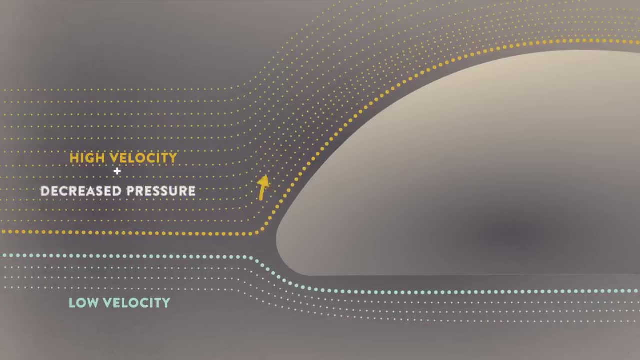 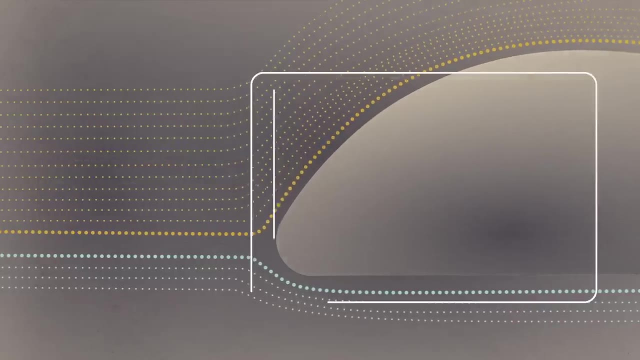 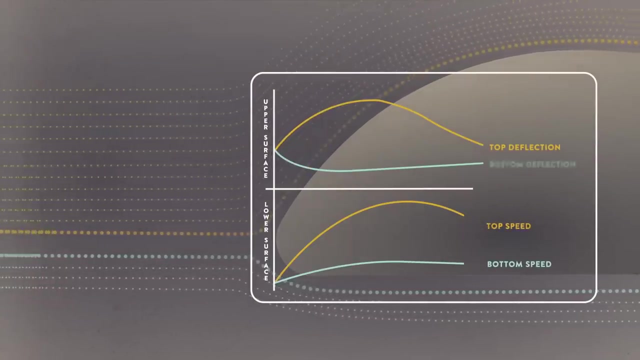 This increased speed is coupled with a decrease in pressure above the wing, which pulls even more air across the wing's upper surface. The air flowing across the lower wing, on the lower surface, meanwhile, experiences less of a change in direction and speed. 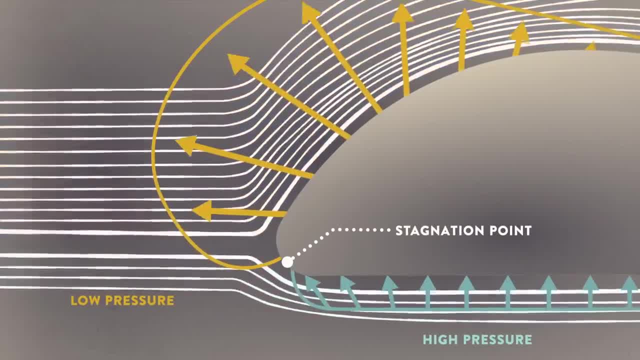 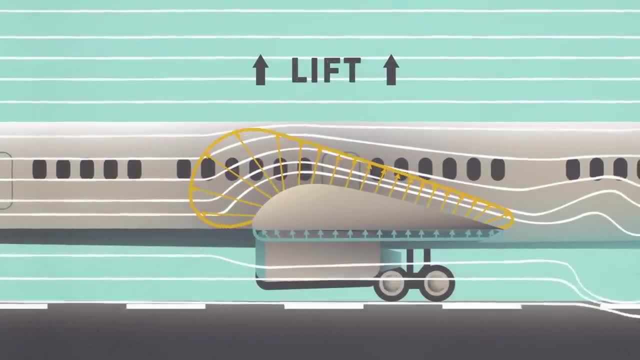 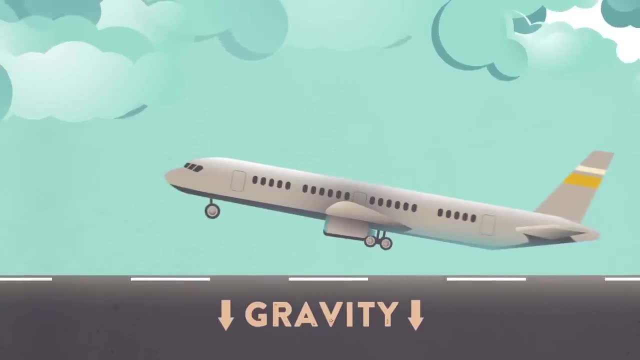 The pressure across the wing's lower surface is thus higher than that above the upper surface. This pressure difference results in the upwards force of lift. The faster the plane travels, the greater the pressure difference and the greater that force Once it overcomes the downward force of gravity. 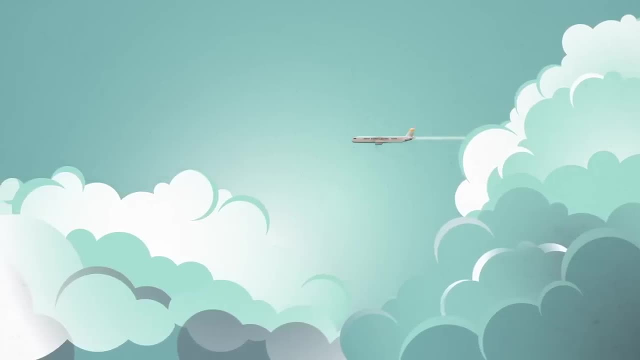 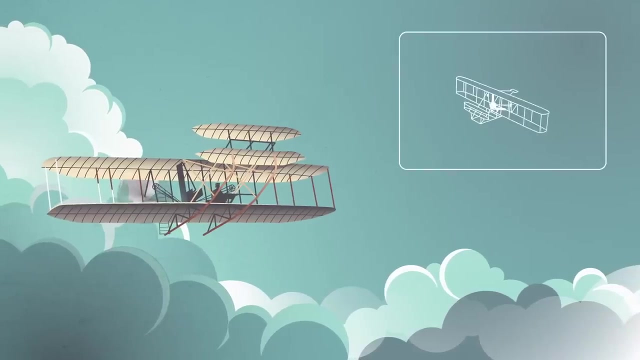 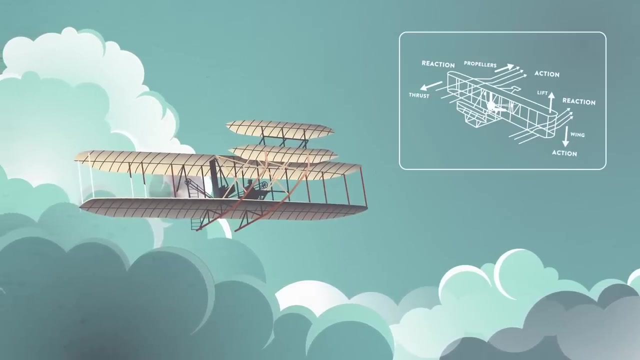 the plane takes off, Air flows smoothly around curved wings, but the wing's curvature is not the cause of lift. In fact, a flat wing that's tilted upwards can also create lift as long as the air bends around it, contributing to and reinforcing the pressure difference. 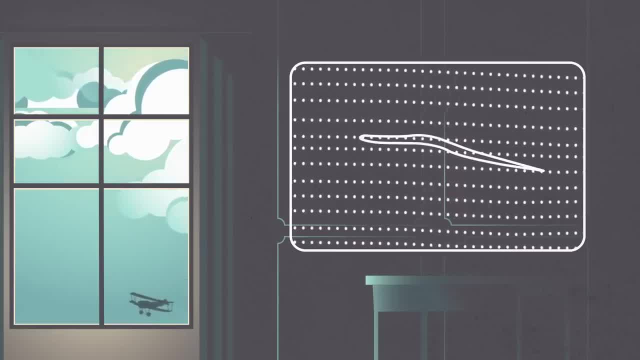 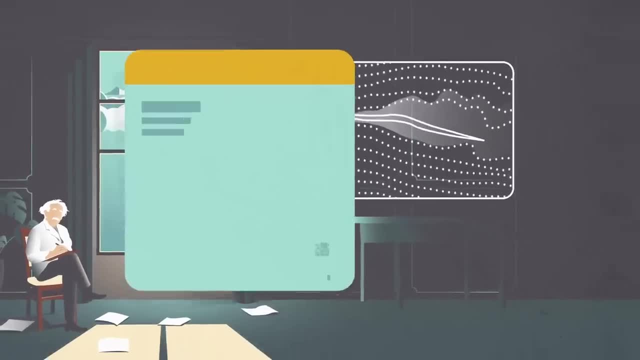 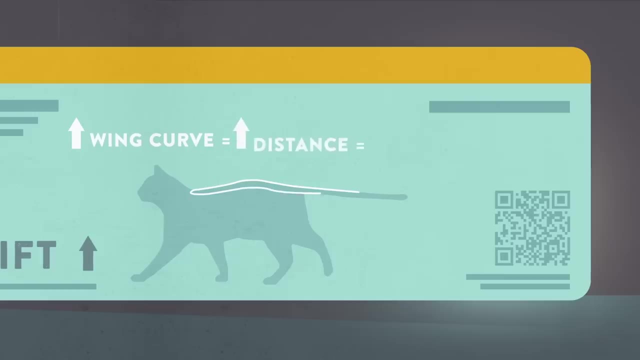 Meanwhile, having a wing that's too curved or steeply angled can be disastrous. The airflow above may detach from the wing and become turbulent. This is probably what happened with Einstein's wing design nicknamed the cat's back, By increasing the wing's curvature. 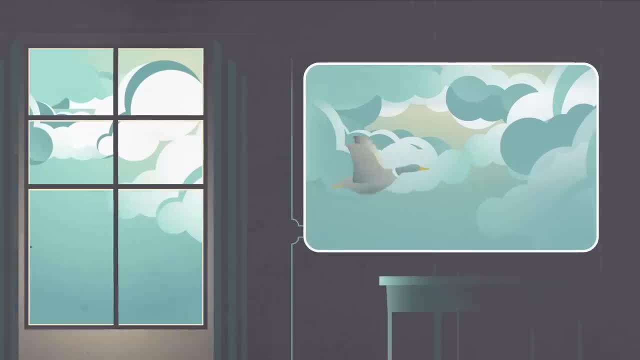 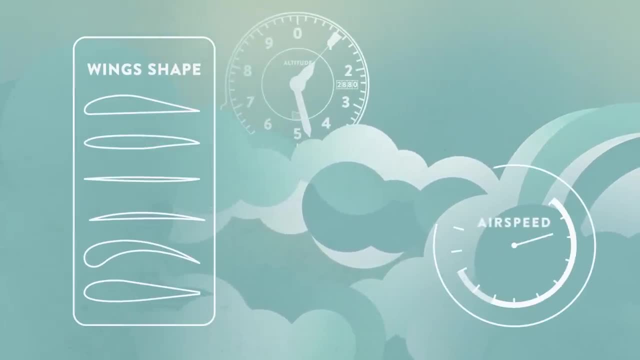 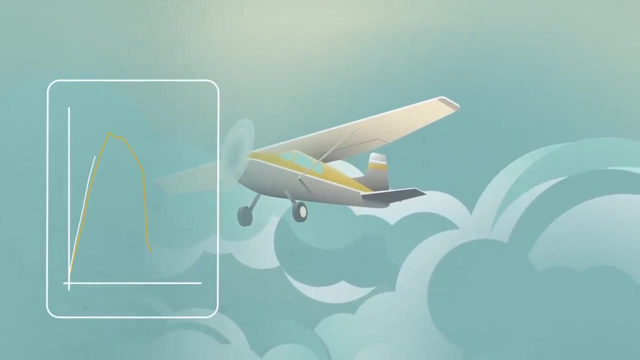 Einstein thought it would generate more lift, But one test pilot reported that the plane wobbled like a pregnant duck in flight. Our explanation is still a simplified description of this nuanced, complex process. Other factors, like the air that's flowing meters beyond the wing's surface. 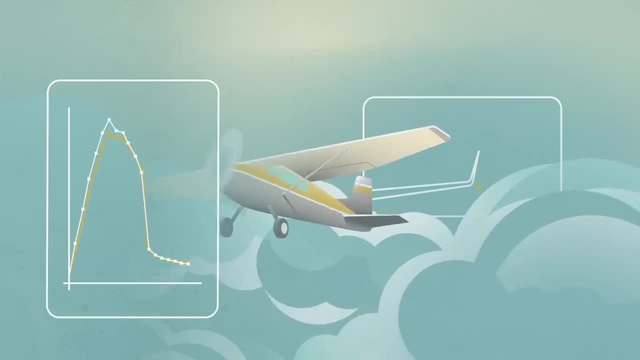 being swept up then down, as well as air vortices formed at the wing's tips, all influence lift, And while experts agree that the pressure difference between the wing's tip and the wing's wing's, wing's wing's lift is the same, and while experts agree that the pressure difference between the wing's tip and the wing's wing's wing's lift is the same, and while experts agree that the pressure difference between the wing's tip and the wing's wing's wing's wing's lift is the same,